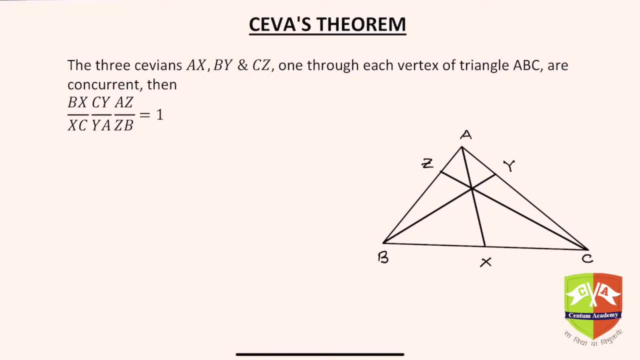 of a triangle, ABC are concurrent, then we get this relationship, This one BX upon XC, into CY upon YA, into AZ, by ZB, is one Interesting, isn't it? So, hence, basically, these are the sides which are being, you know, cut by the CVNs, So the product of each in a cycle, So BX upon XC. So, if you see, 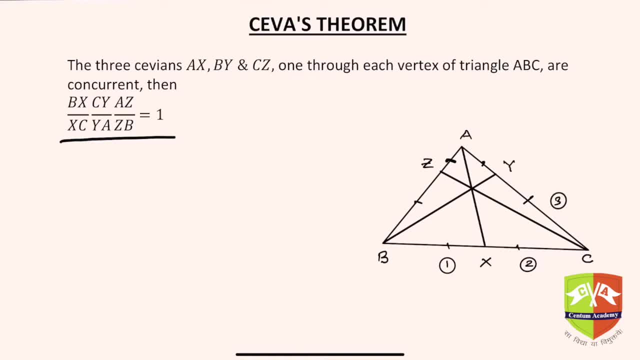 this one by two, into three by four. So three by four are not the numerals, but the you know. so I'm just labeling these sides- and then five by six. if you multiply all of them, One by two, into three by four, into five by six, gives you one. So that's what this particular theorem says. Now let's try. 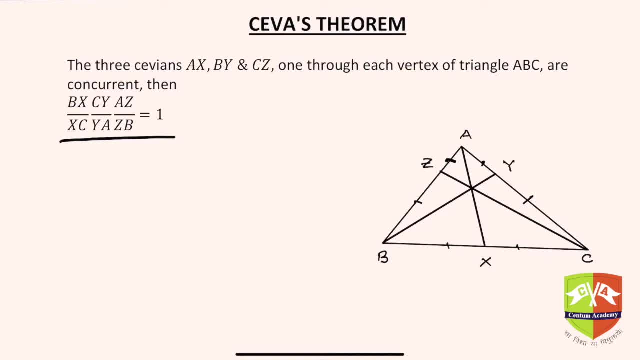 to prove this theorem. Okay, so how to go about the proof? So hence, in this concept, in this particular theorem, we will be using the area Concept, right? So, area of two triangles with the same base and between same parallel or with same altitude. The two areas are equal in that case. So hence, if you see, let's take BX and XC. So, if you 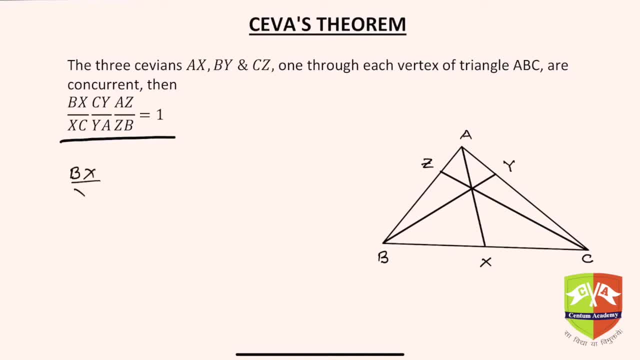 see BX by XC. If I take this ratio, what is BX by XC ratio? It's nothing. but I can write half into BX, into, let's say, H. What is the H BX into H? Okay, so H you can think of. let's say there is a. 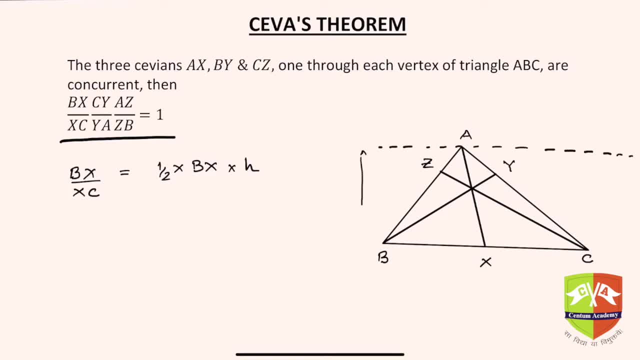 parallel line and the distance between these two is H. So half into base, into height, divided by. can I not write this as half into XC, into H? Okay, let me write it once again, So it is one by two into. let me put it in brackets so that: 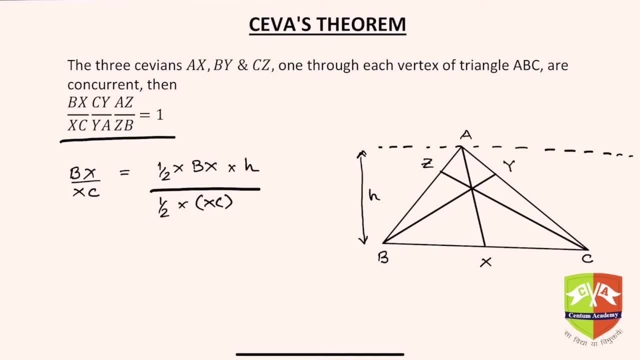 you know you don't get confused it with multiplication sign XC into H. Can I write that? because half and H are common in both numerator and denominator. Now, if you see closely, this particular thing is nothing but area of triangle A, triangle A, B, X, right, and the denominator is area of triangle A, X, C, A, C, X. let's say Okay. now let's say the three. 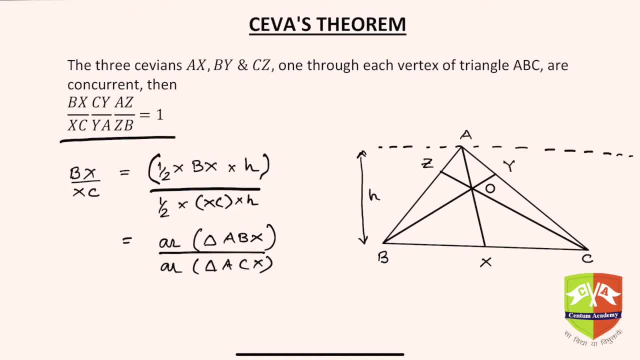 the point of intersection is O or point of concurrence is O, So the same thing can be written about O B, X and O X C. So if you see again this, it will be nothing but area of triangle O B, X divided by area of triangle O C X. Why is this? Because if I write it here in brackets, what is O B, X? 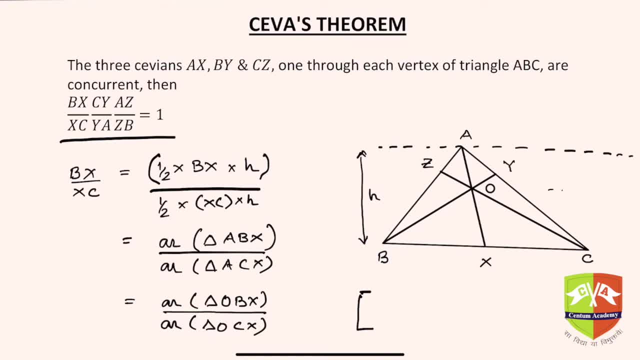 guys, area of O B X will be- let's say the height is again some other- H 1. then O B X area is half into B X, into H 1 and if you see the denominator, half into C X, into H 1, isn't it same? So H 1, H 1 goes. 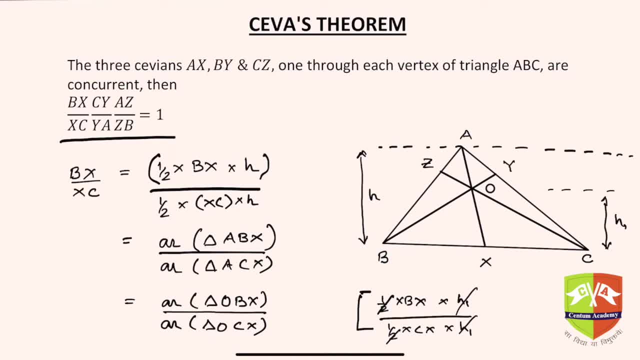 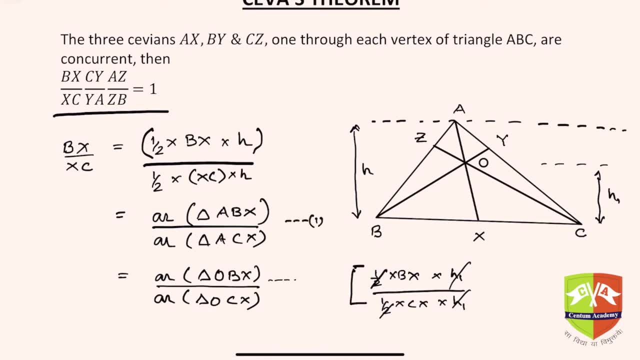 down. So this ratio also is equal to B? X upon X C. That's important, Okay. so if you see from this one and two, so both are equal to B X upon X C. Let me write like that: B X upon X C, isn't it? B X upon X C. 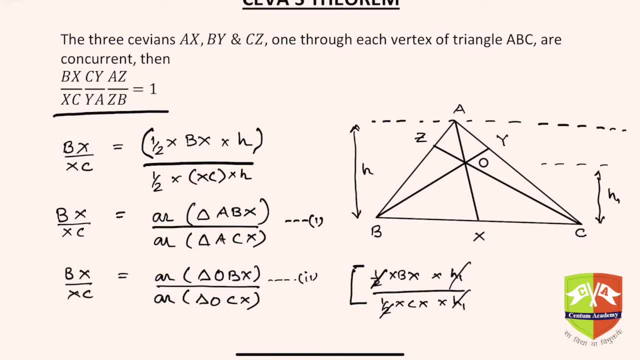 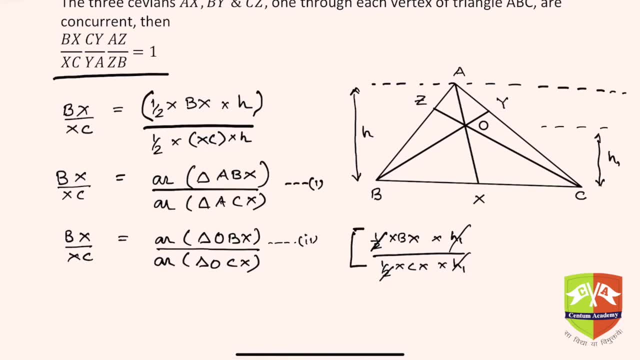 both are equal. Now, if two ratios are equal, so they are correct. difference of numerator and denominator. So you know: componendo and dividendo. So hence I can write this by componendo or only dividendo: B, X by X. C is equal to area of triangle A- B X, minus area of triangle O, B, X. 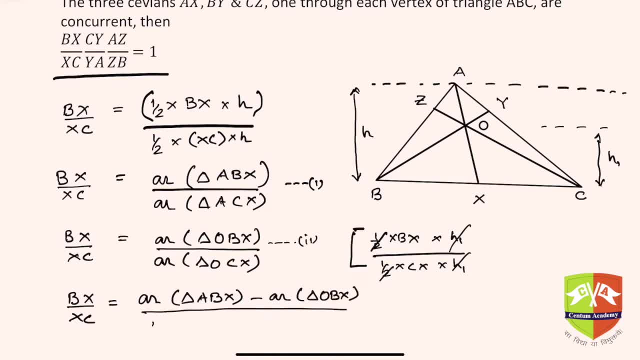 divided by area of triangle O C X minus area- sorry, not this one- will be A C X minus area of triangle O C X. clearly right. Why am I saying this? because if A by B is equal to C by D, then if this will also be equal to A minus. 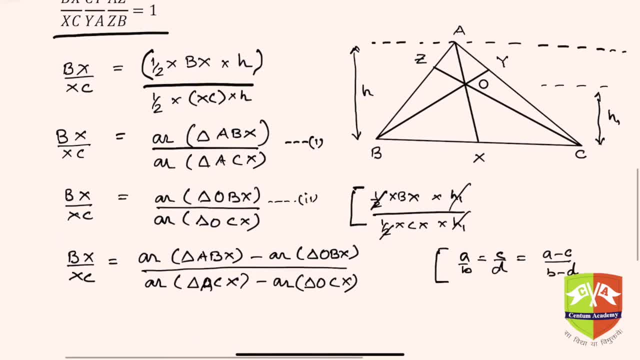 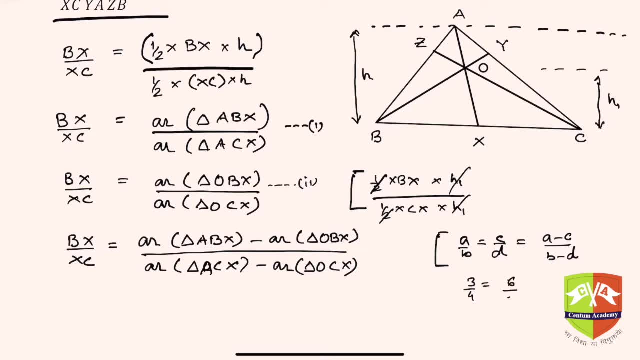 C divided by B minus D, you can check. Let's take an example. So 3 by 4 is equal to, let's say, 6 by 8, isn't it? 3 by 4 is equal to 6 by 8.. So if you do, the difference, 3 minus 6 by 4 minus 8 is equal to. 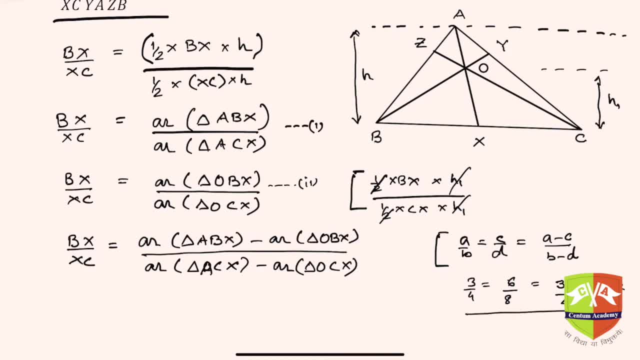 3.4.. All are same. This is just for explanation purposes, nothing else. So we get this relationship, guys, A B X upon X C. is this? Now, if you look closely to the figure in the figure, area of A B X minus area of O B X will be nothing but this shaded region, Right? So hence I can write now. 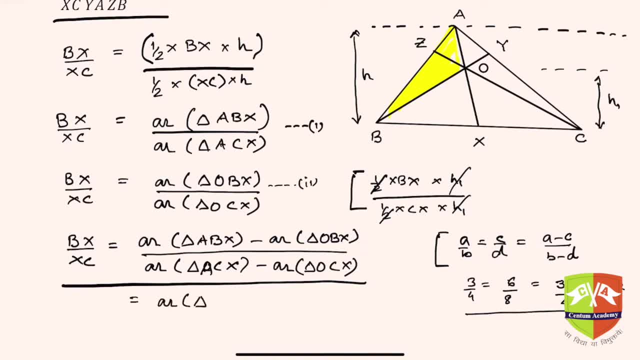 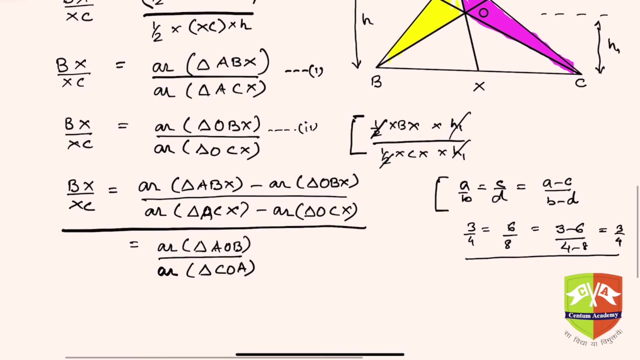 this as area of triangle A O B And in the denominator, If you see, this is nothing but A, C X minus O C X. is this particular area? right? it's particular area. So hence You can write it as area of Triangle triangle A O C or C O A, isn't it So what we infer, we we got B X upon X C- is equal to area of. 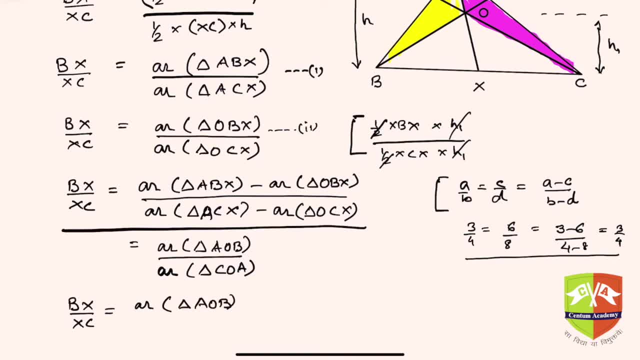 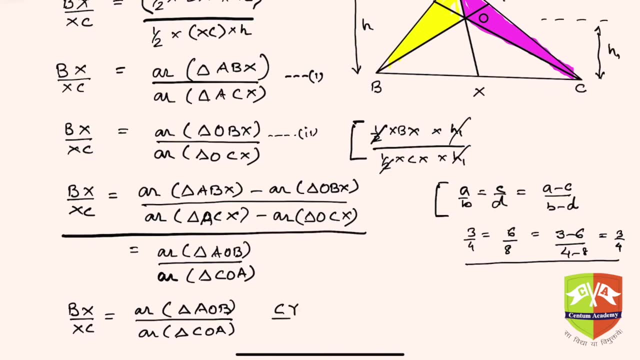 A triangle AOB, divided by area of triangle COA. and similarly, if you repeat the process for the other three other two CV n's, you will get C Y upon Y a. okay, C Y upon Y a will be equal to area of C Y upon C. Y upon Y a will be nothing but. 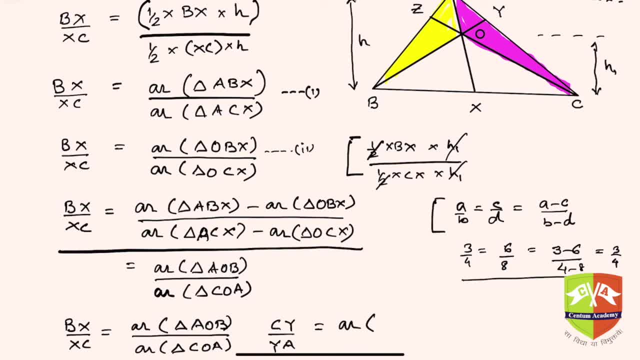 area of BOA, or rather C Y is first right, so hence a heart. so it will be triangle BOC, BOC, divided by area of triangle AOB. triangle, AOB, right. you can check in the same process. you will get the same result and similarly you will. 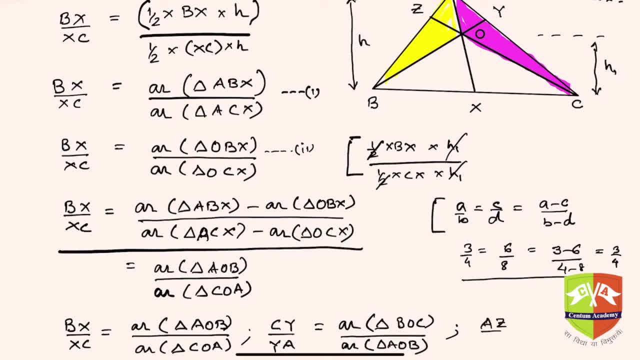 get a Z by Z B. if you see this, a Z by Z B will be a OC triangle triangle, COA. this is area right area of COA divided by area of COB or BOC, right triangle, BOC. so this is what you get now if you multiply all the three, these three. so hence, what will you? 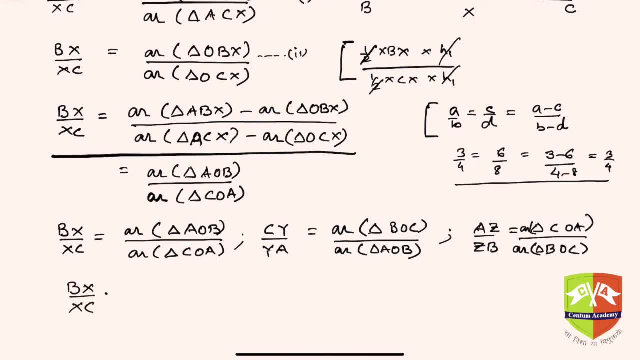 get LHS. multiply all the LHS together, so B, X by X, C into C, Y by Y, a into a, Z by ZB, will be equal to area of triangle AO- B divided by area of triangle COA, into area of triangle BOC divided by area of triangle AOB and. 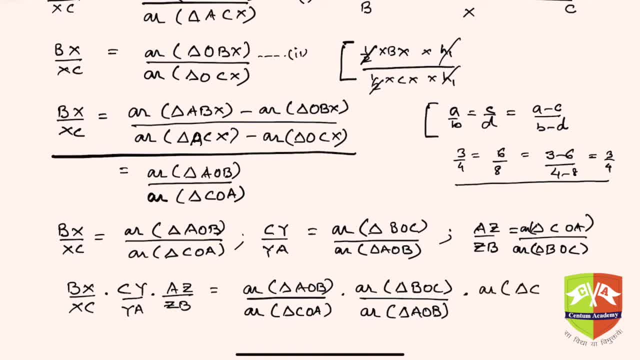 this is multiplied by area of triangle coa, divided by area of triangle boc. now all the areas are greater than zero in this case, so hence we can cancel all of them. boc case goes, coa goes, hence this is one, hence we prove the result right. so ax by xc, into cy, by ya, into az, by zb, right is equal. 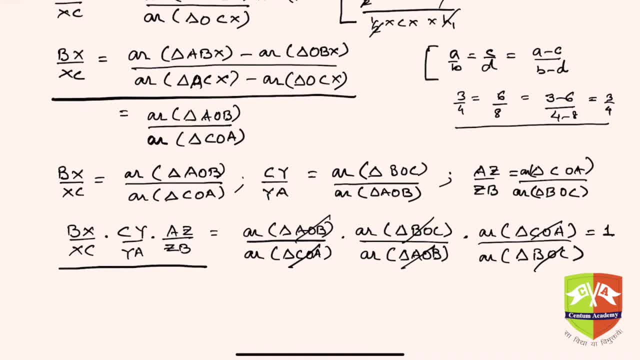 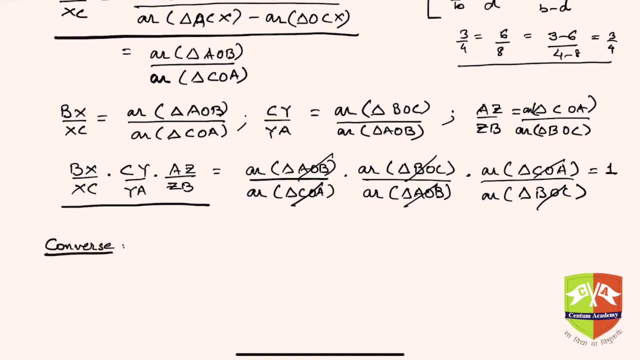 to one. so this is what we needed to prove. in fact, converse is also true. that means converse. if you just check converse, what will be the converse of this? so in a given triangle, i can word it out like that: in a given triangle, given triangle, if, if bx by xc is and into cy by ya, into um. 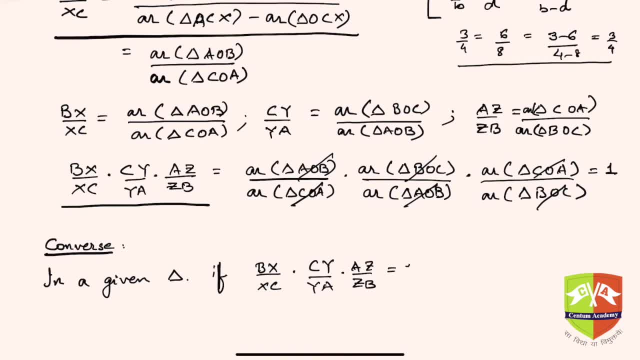 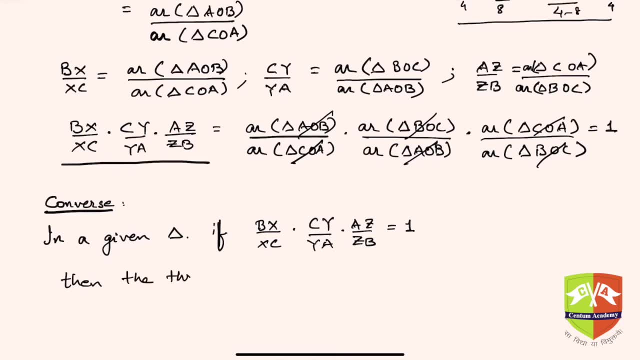 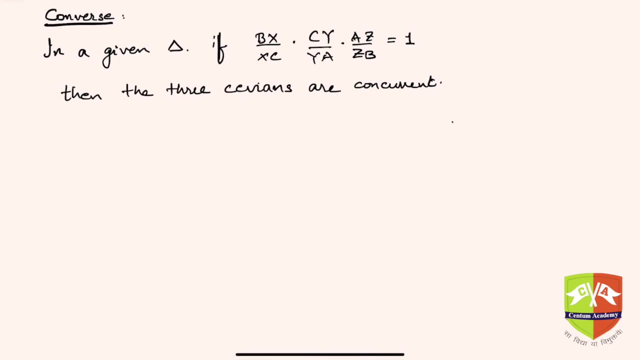 a, z by z, b equals one equals one. then then the three cvns: cvns are concurrent, cvns are concurrent. this converts, this is the converse, and you can prove it easily again. so in this case, what will we do is, let's say: this is a triangle, abc and 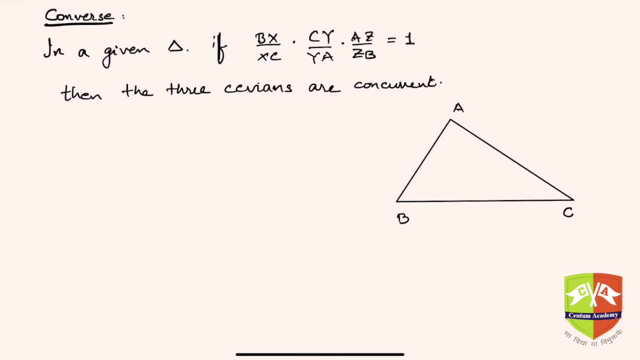 bx by xc, by xc into cy, by ya, into c, z or apx cz, and then we have what we call the remembers. when compared to second time, this speaking of before which happens, is this be? this possibility does not work in. it does not work in this case, per-a. when we tile this plan, then let's say two cv's, let's, let's try with it two cv's first. so let's say by, and this one cz, okay. and let's say this point is x and it is given that what is given. so bx by xc into cy by ya xc, and then cz by y. 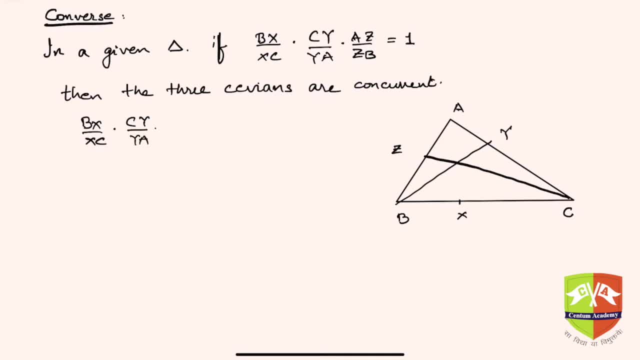 and let's say, this point is x and it is given that what is given, so bx by xc, into cy, by ya, into y, a, into az, by zv, is equal to 1. it's given, isn't it? it's given. so, let's say, at least two cvns will. 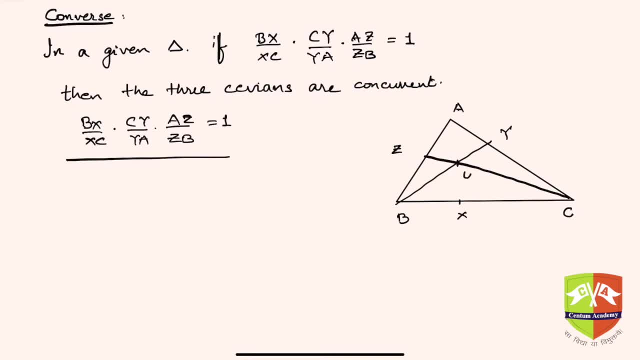 definitely intersect, if not all three. so let's say this: intersection is o, point, point of intersection is o. then what do we get? uh, we know. um, then, uh, by cvn, cvs, cvas theorem, i can, let's assume that there is a cvn which is uh going on x, but now this is very closely placed. so let me. 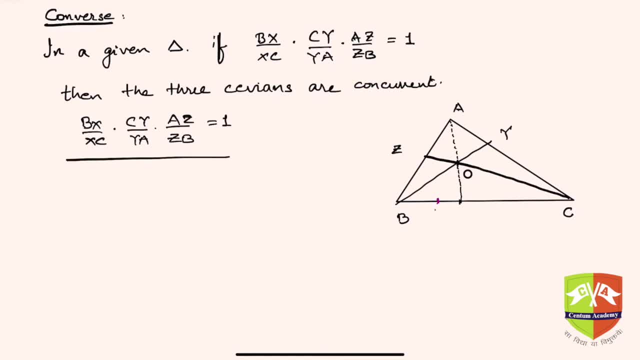 uh, remove this point and let's say: this is the point x. okay. and by cvas theorem, let's say: we'll definitely get one cvn which passes through a, o, and let's say: this is x, dash. so by cvas theorem, by cvas theorem, what do we get? 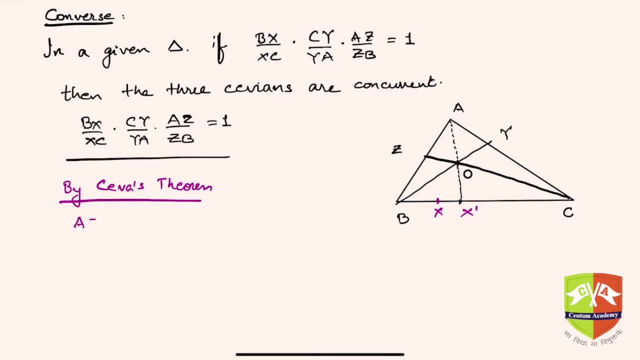 v. get this az by zb into um, bx, dash by x, dash, c into cy by ya is equal to 1. but if you see, what was given given was this: so hence from let's say this is 1 and 2 from 1 and 2 from from 1 and 2, what can we infer? we can infer: